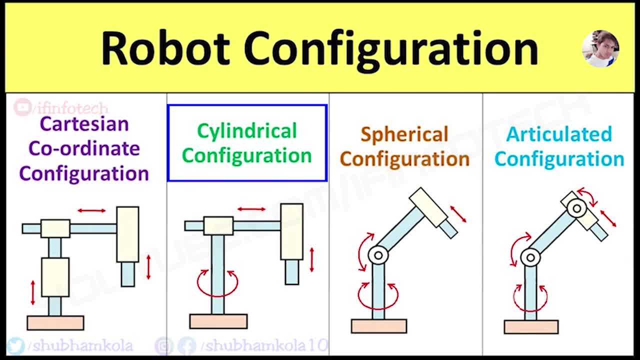 The Next is cylindrical configuration. As you can see in this video, the robot requires In this figure it consists of two prismatic joints perpendicular to each other and one revolute joint mounted on rotary axis. Difference with Cartesian configuration is one prismatic joint is replaced by revolute. 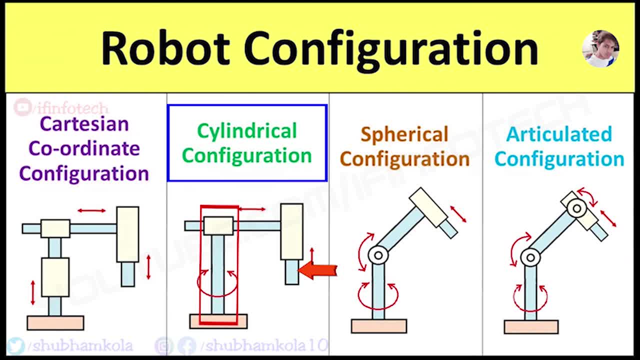 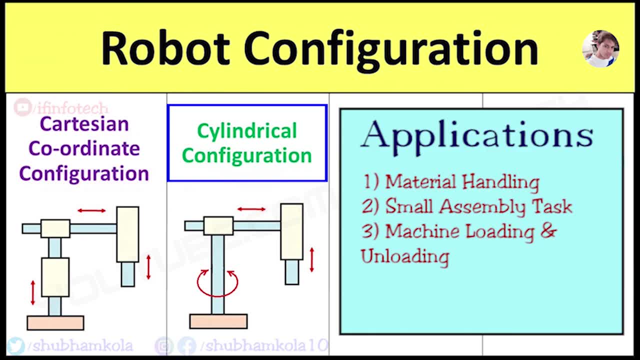 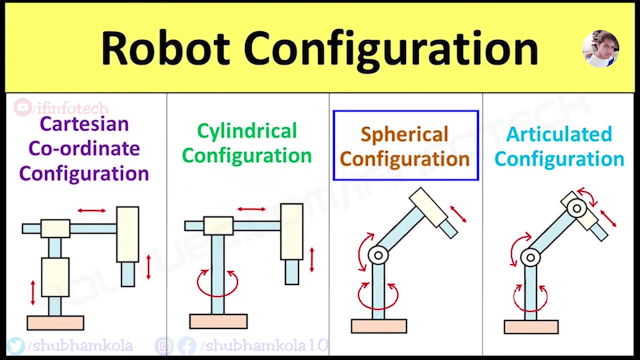 joint Vertical column carries arm assembly that move up and down. It also rotates about column. The cylindrical configuration is used in motor handling, small assembly, task machine loading and unloading. Next is spherical configuration, It also called as a polar configuration. 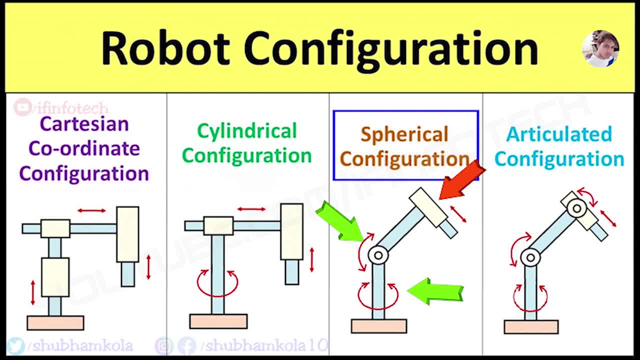 It has one prismatic joint and two revolute joint. First rotary movement occurs about a vertical base axis, while second rotary movement is of pure point about horizontal axis. Prismatic joint moves wrist rapidly in and out. This configuration allow robot to operate in horizontal axis. 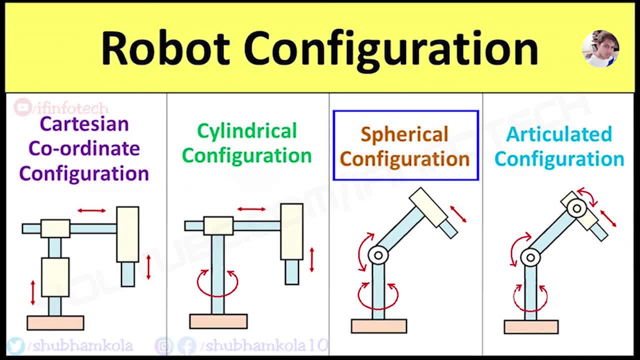 Next is spherical work volume. It provides larger work envelope than Cartesian or cylindrical configuration. Next is articulated configuration. It consists of three revolute joint and one prismatic joint. When arm rotates about all three major axis, result configuration is articulated configuration. It is also called as joint arm configuration. 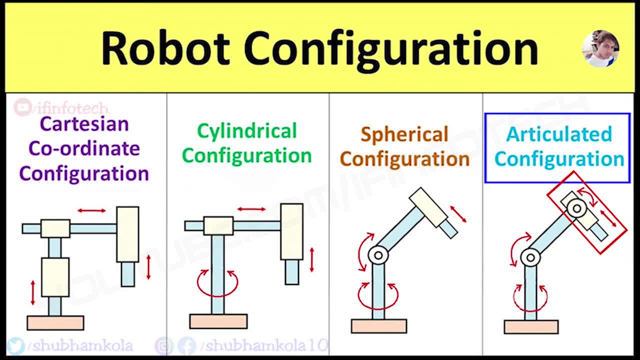 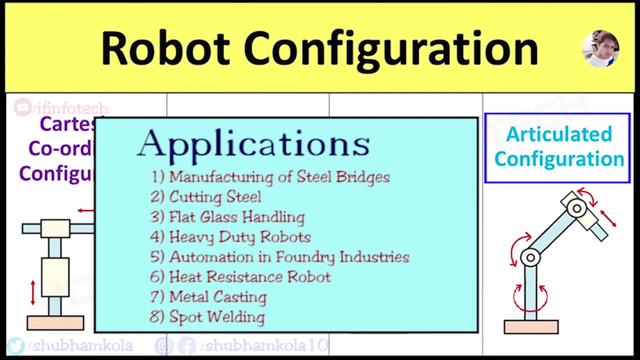 The arm of this configuration look like a human arm. It has two rotary joints, shoulder and elbow, about their respective horizontal axis. The third rotary joint is about vertical base axis. It is used in manufacturing of steel bridges, cutting steel, flat glass, handling heavy. 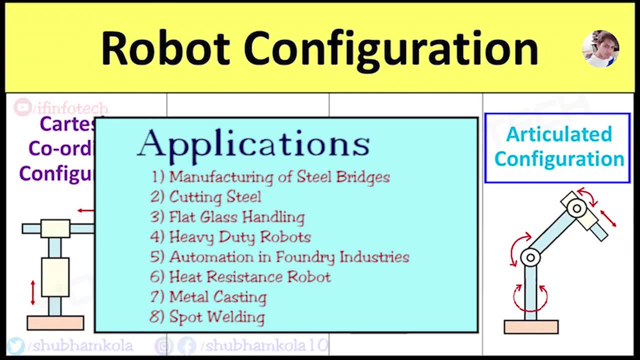 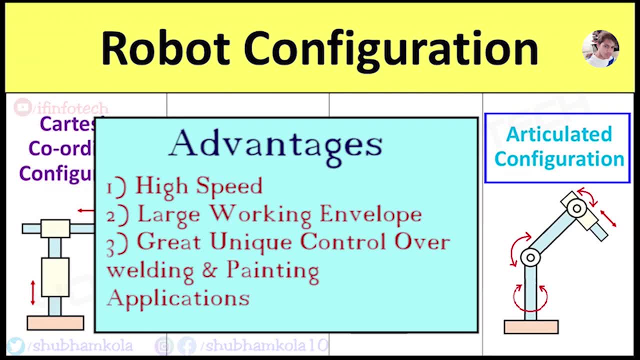 duty robot automation in foundry industries: heat resistance robot, metal casting, spot welding. Now you see the advantages. This robot has high performance, This robot has high performance. This robot has high performance, It has high speed, It has large working envelope. 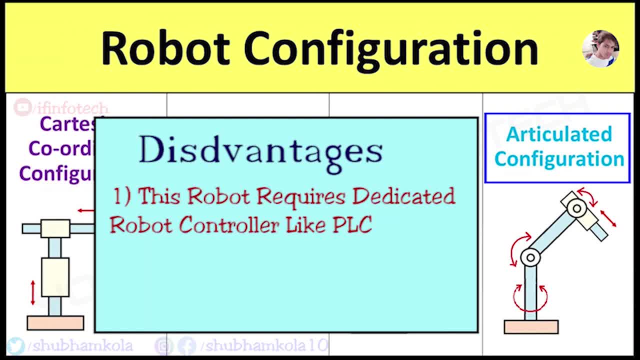 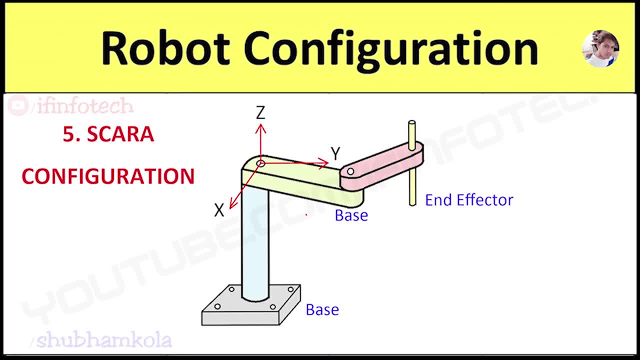 Great, unique control over welding and painting applications Here. the only disadvantage is it requires dedicated robot controller like PLC. Next is SCARA configuration. It is a special version of a jointed arm robot whose shoulder and elbow joints rotate about vertical axis instead of horizontal.